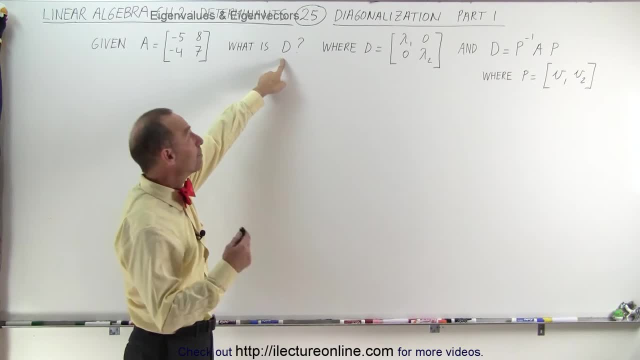 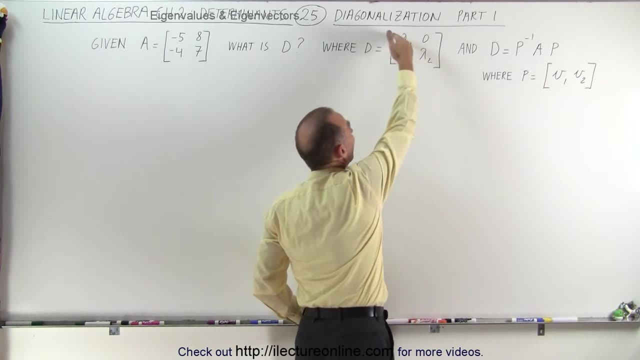 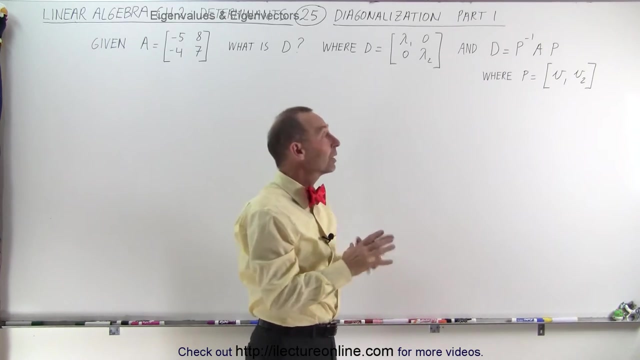 the elements. We're trying to find the diagonalized matrix. and the definition of the diagonalized matrix of A is that it's simply the eigenvalues along the diagonal and zeros everywhere else. You may say, well, why would we want to do that? Well, it turns out that you can also find the 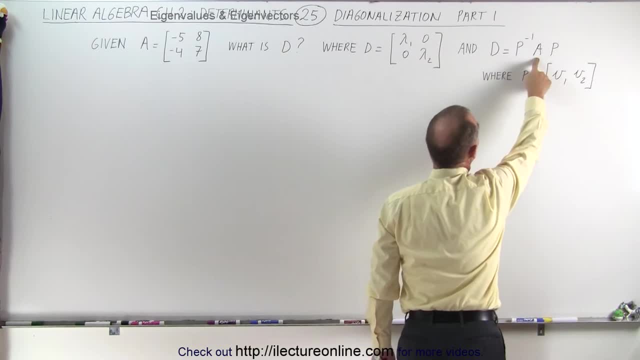 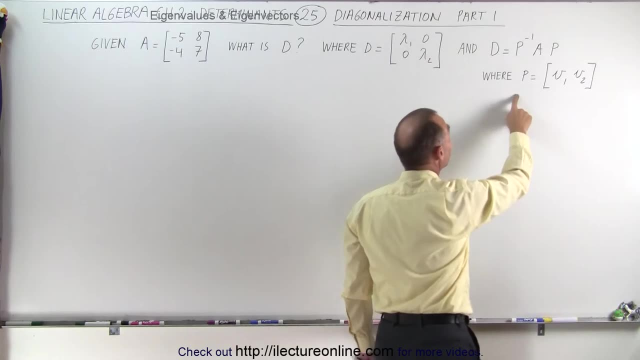 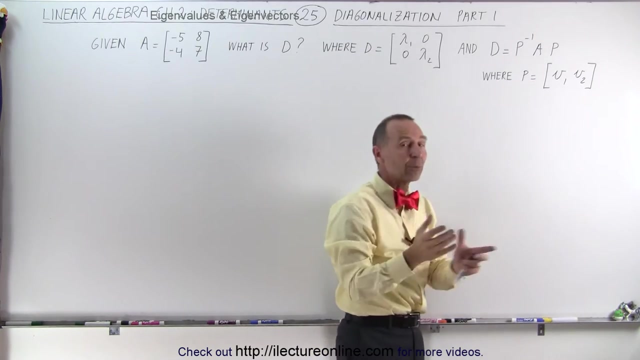 diagonalization of the matrix. by taking the matrix here, multiplying, it times the p matrix and the inverse p matrix. The p matrix is defined as the matrix that's made up of the eigenvectors corresponding to the two eigenvalues. So there's a nice relationship there, and then later on we'll also find out how we can use the. 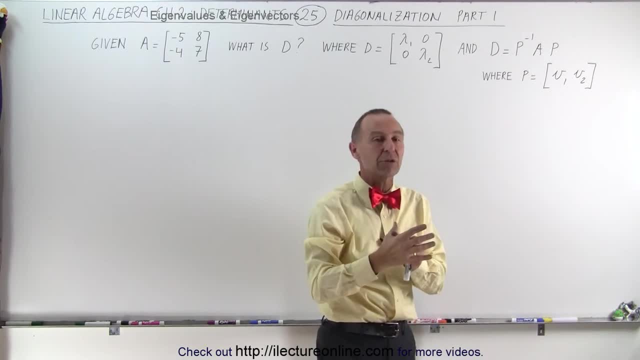 diagonalized matrix to find the power of a matrix like A squared, A cubed or A to the hundred power. Imagine trying to find A to the hundred power using a calculator when there's an easier method to do that. But we need to know how to diagonalize the matrix first. So let's start with that. 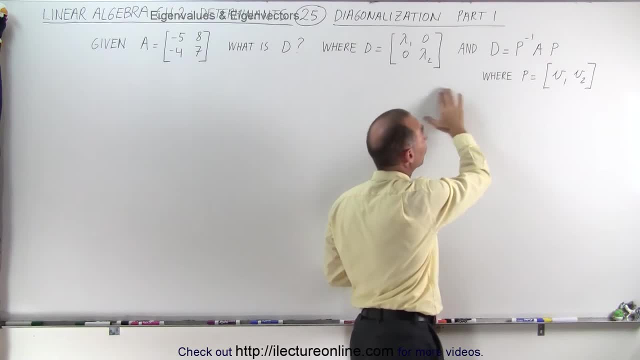 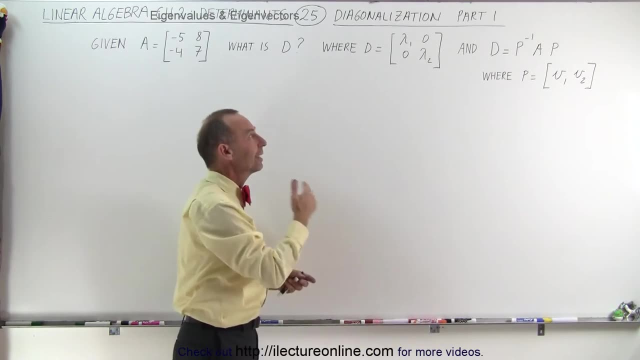 principle first, and then we'll see how we can find that eigenvalues, In other words, find the diagonalized matrix using the diagonalized matrix, this principle here, and then we'll learn how to find the power of a matrix, again using the diagonalization method. So first we need to find the diagonalized 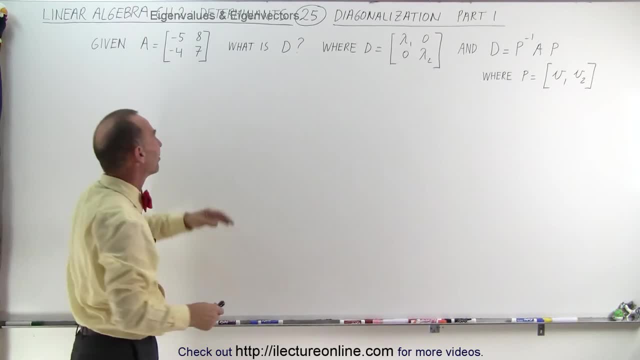 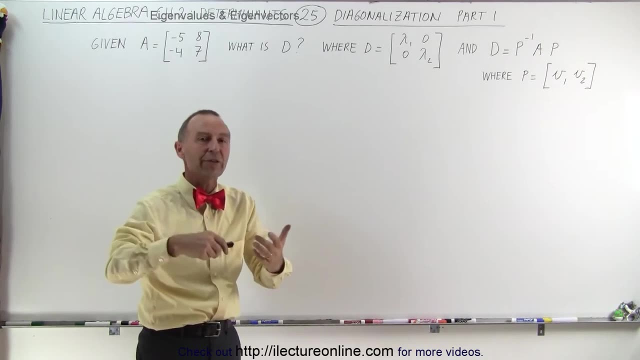 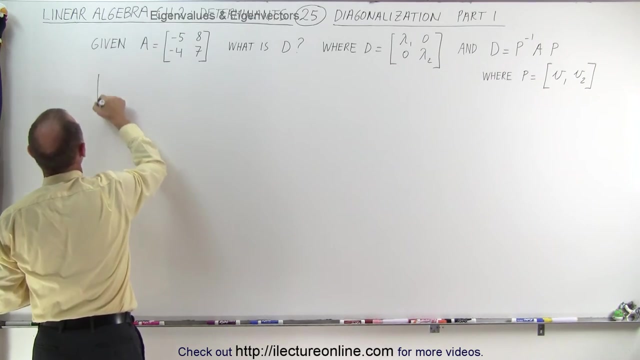 the diagonalized- whoo- that's a hard word to say, isn't it? diagonalized matrix of A by finding the eigenvalues. Now we know how to find eigenvalues in the old-fashioned way, so let's do that for some practice. We're going to turn this into determinant and subtract the eigenvalues. 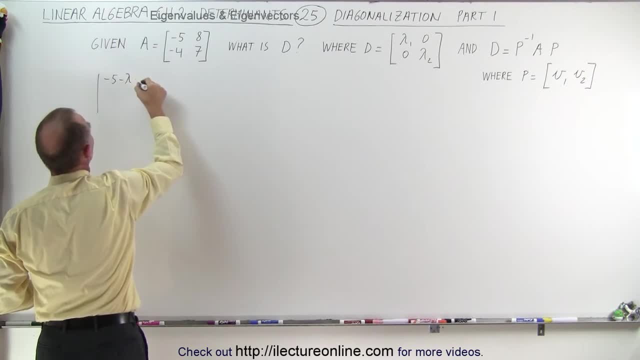 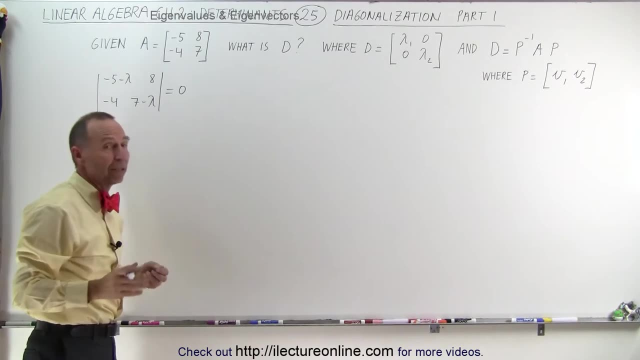 from the diagonal here. So minus 5 minus lambda, 8 minus 4, 7 minus lambda, and we're going to set that equal to 0.. That's the method to find the eigenvalues We cross. multiply these and minus the product of those minus times a minus. 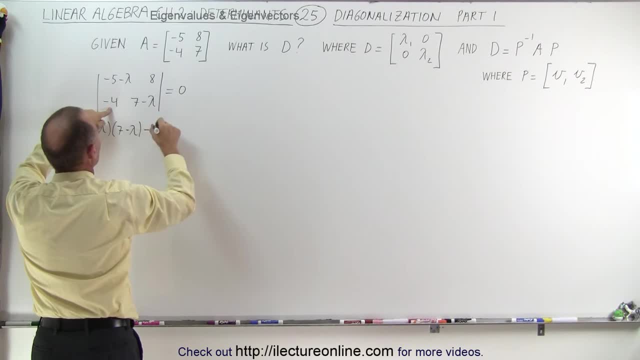 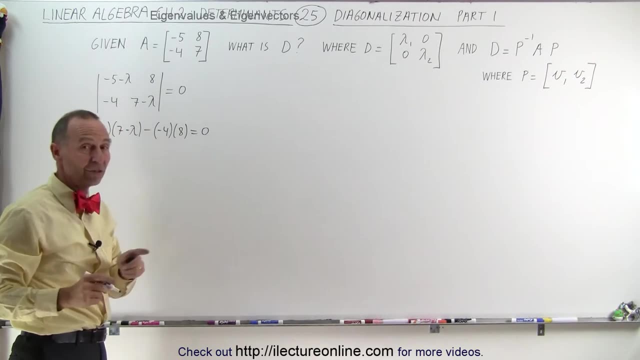 that becomes a plus 4 times 8, or I can simply show you how to do that. I'll show you what it looks like. so it's minus, a minus 4 times 8, and we set that equal to 0.. Now we have to solve this for lambda, because this is a quadratic. 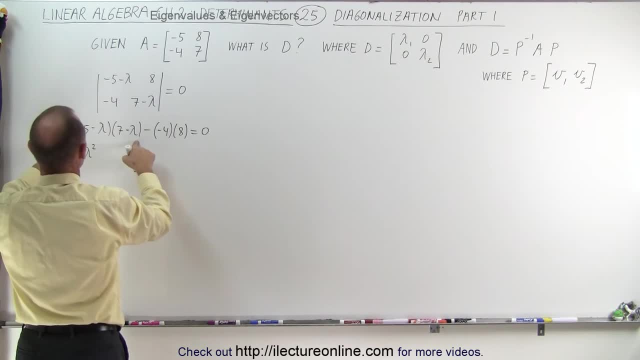 equation: Lambda squared plus 5 minus 7, that's minus 2 lambda and a minus 35 and plus a 32 is equal to 0.. This is: lambda squared minus 2. lambda minus 3 equals 0, and factoring this we get lambda minus 3. lambda plus 1 equals 0 and that means. 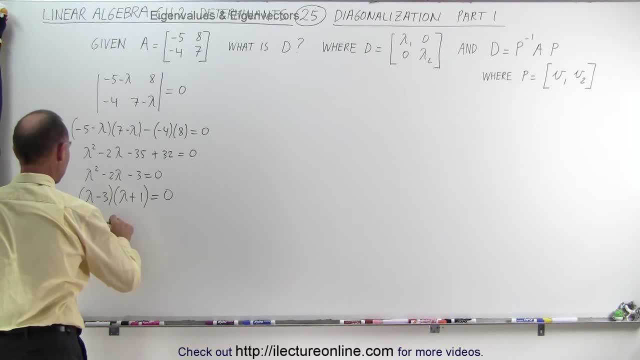 that we have two eigenvalues. We can say that lambda sub 1 equals minus 1 and lambda sub 2 equals 3.. Those are our two eigenvalues. That means that our diagonalized matrix will look as follows: d is equal to 2.. 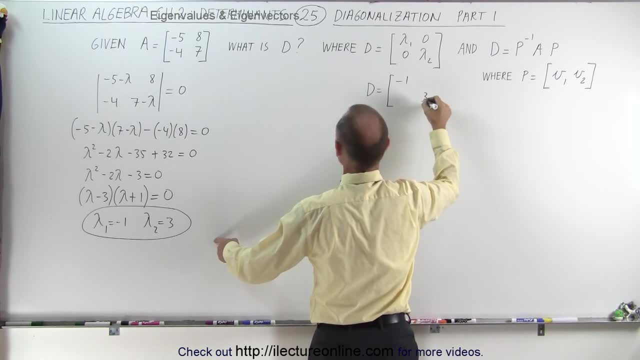 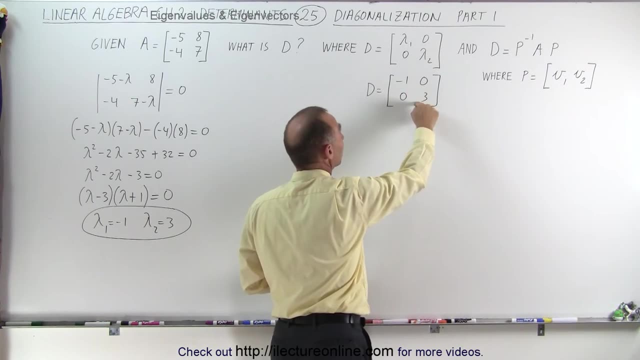 d is equal to 2.. We have minus 1 and 3 along the diagonal and 0, 0 everywhere else. And you may wonder: well, would it matter if I put the 3 up there and the minus 1 down here? and that would make no difference at all. 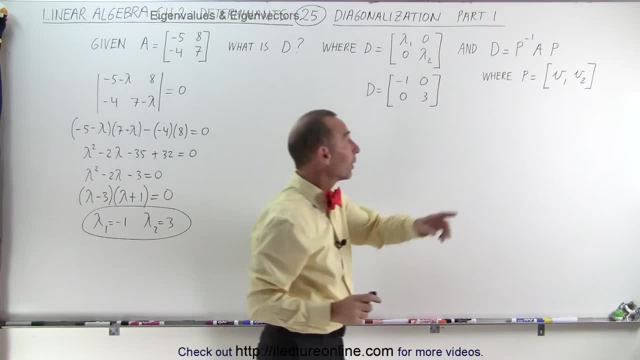 So what we're going to continue doing now is because we're also going to later want to find out the diagonalized matrix using this methodology. here we're going to need to find our eigenvectors corresponding to those two eigenvalues. So, starting with, let's 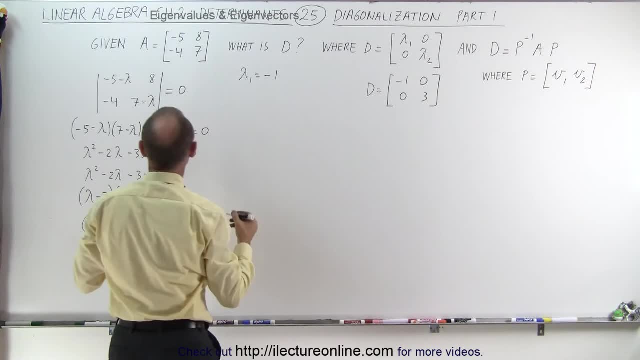 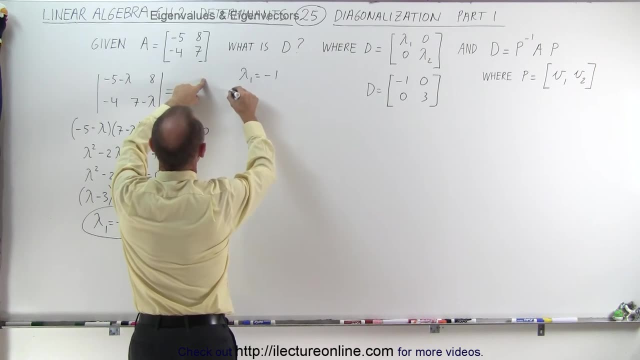 say lambda 1 equals 2. lambda 1 equals negative. 1. To find the eigenvector, we're going to subtract the negative 1 from the diagonalized diagonal elements, Minus 5, minus a, minus 1, which is plus 1.. 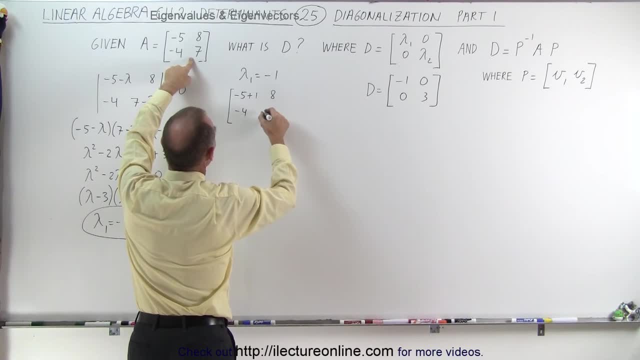 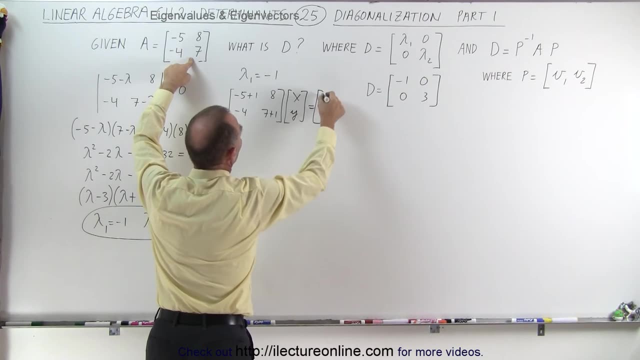 8 minus 4.. 7 minus a minus 1, which is 7 plus 1.. Multiply times x and y and we get the zero matrix That will allow us to find the first eigenvector corresponding to that. d is equal to 0.. 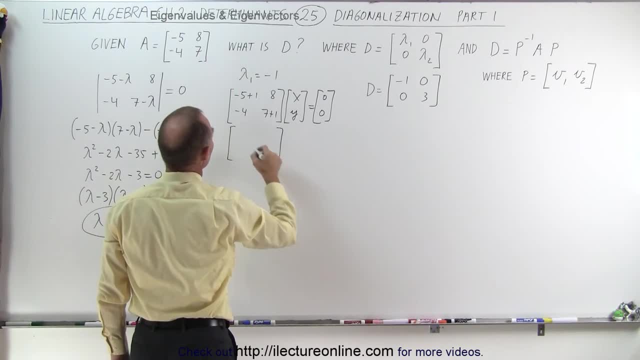 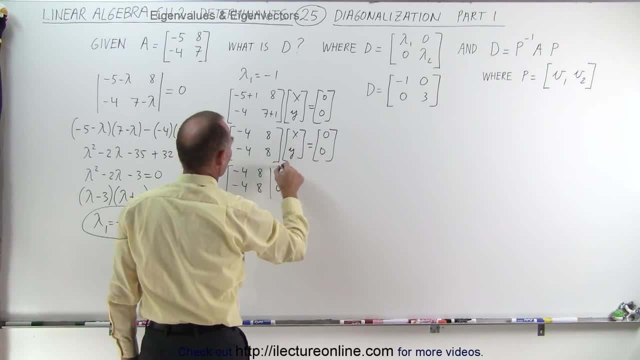 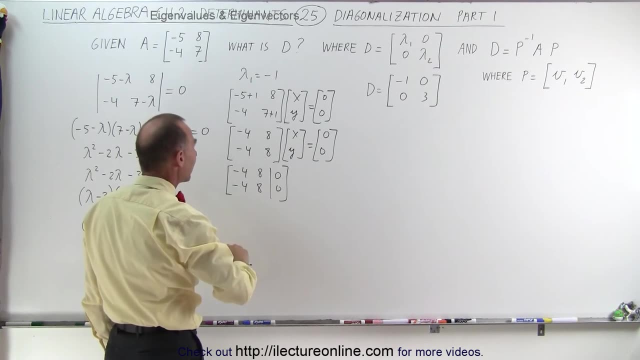 0, 0.. Now we place that into the augmented matrix: Minus 4 minus a, minus 4 minus 8, minus 4, minus 8 minus 0.. Of course it's quite obvious at this point that these are duplicates. 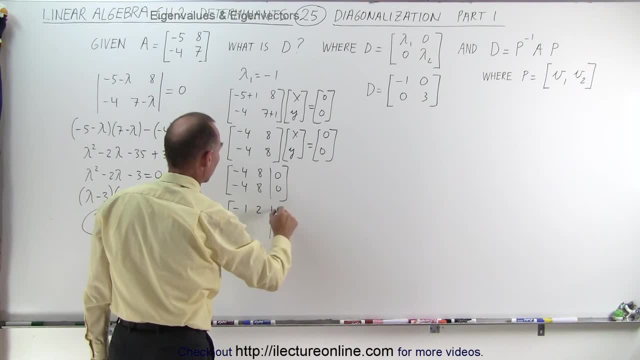 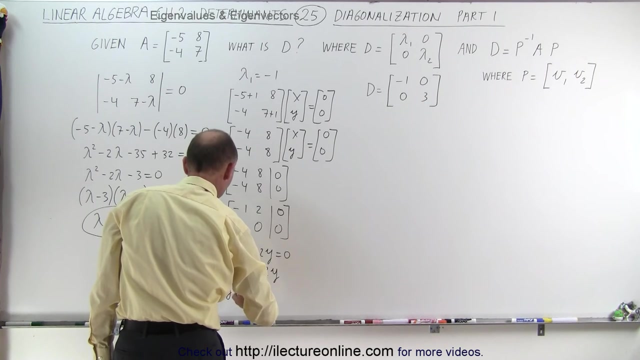 So we can get rid of one of them, and this can then be written as a minus one, two, zero, zero, zero, zero. that's a zero, which means that minus x plus two y equals zero, or x equals two y, which means when y is equal to one. 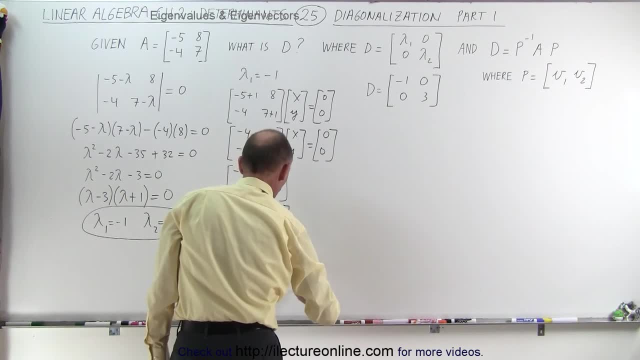 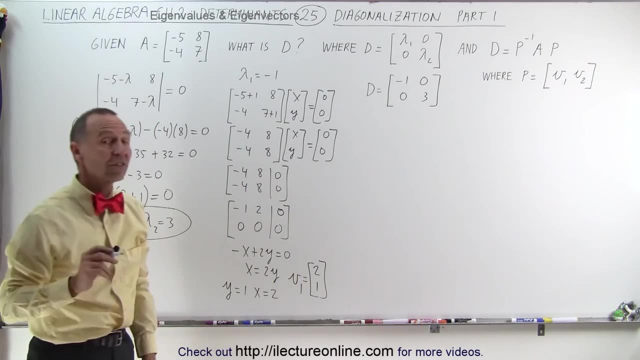 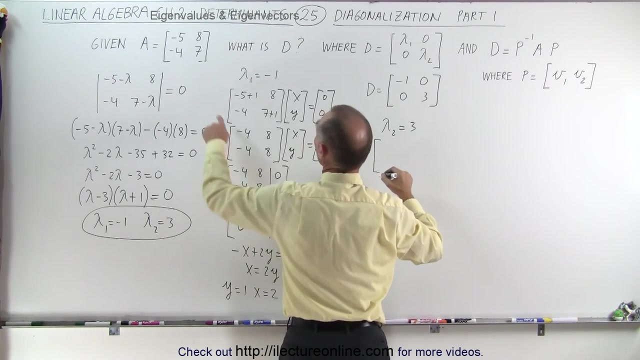 x is equal to two and the eigenvector v1 corresponding to this eigenvalue is equal to two and one. let's do this again with the second eigenvalue: lambda sub two equals three, which means we take minus five minus three and eight negative four seven minus three. 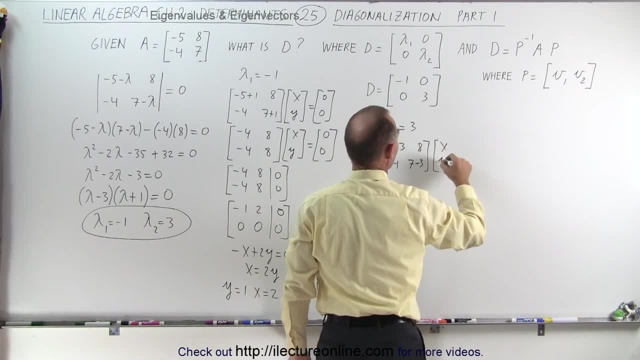 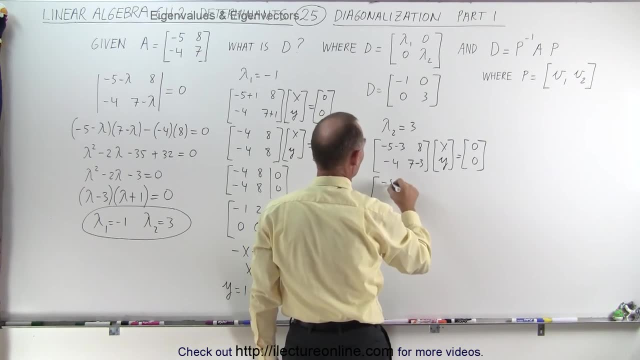 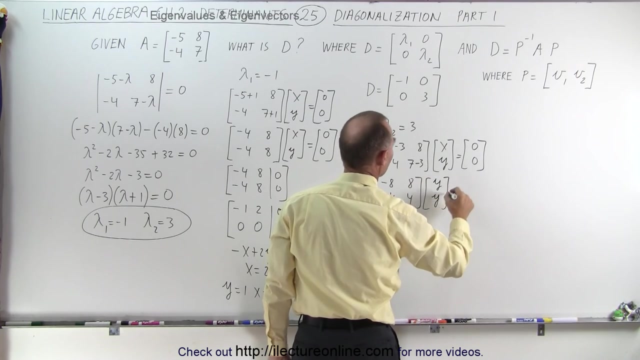 multiply the times, the eigenvector x, y, and we should get the zero vector, zero, zero, which means that minus eight and eight minus four and 4 times X, Y gives us the zero vector and again it becomes quite obvious that we end up with duplicate rows, which means that we end up with minus 8 and 8. 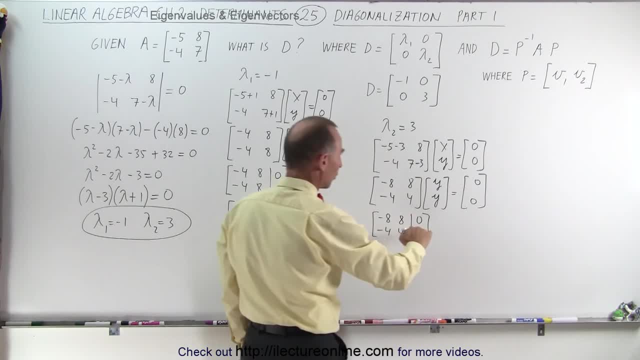 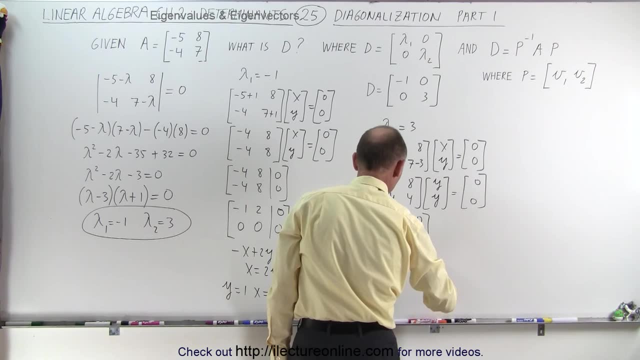 if we draw the odd 4: 0, we get rid of one of the rows and divide the top row by 8, we get negative 1 1 0, 0 0 0, which means that minus X plus Y equals zero or X equals Y. 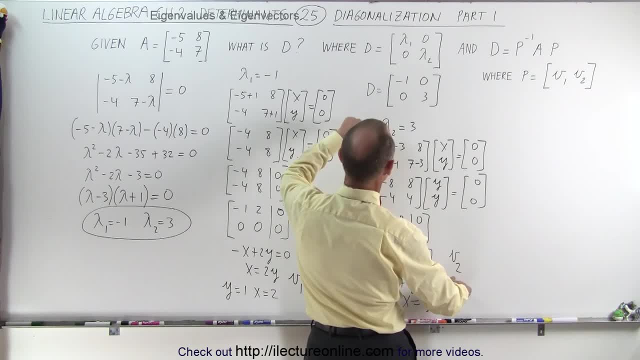 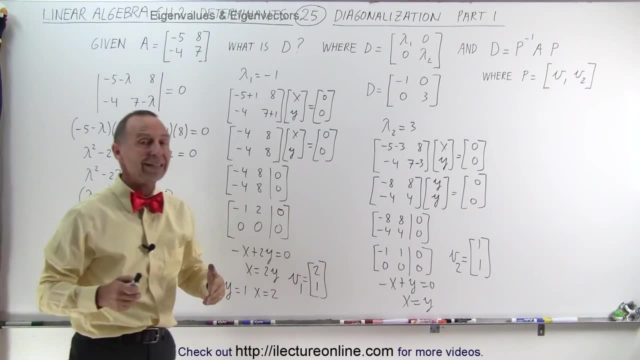 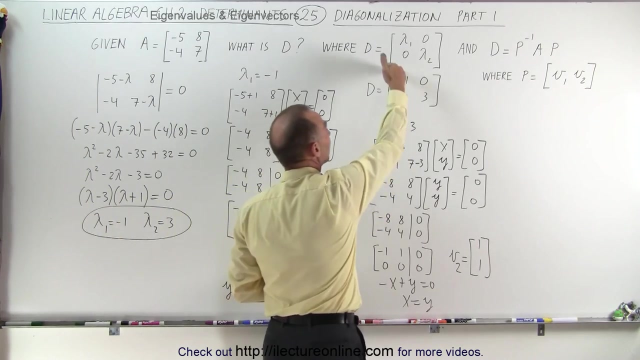 which gives us the second eigenvector corresponding to this eigenvalue of 1 and 1. So now we see that to find the diagonalized matrix, one way to do that is to go ahead and find the eigenvalues. plug the eigenvalues in the diagonal here. 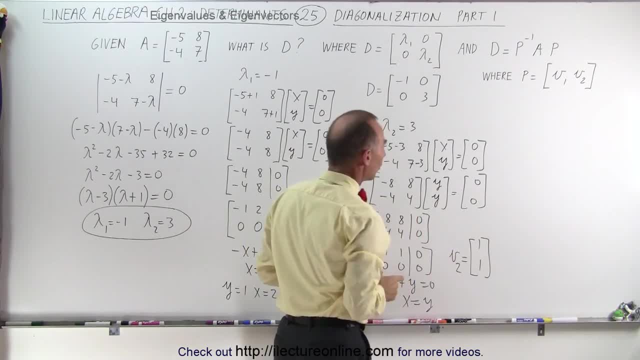 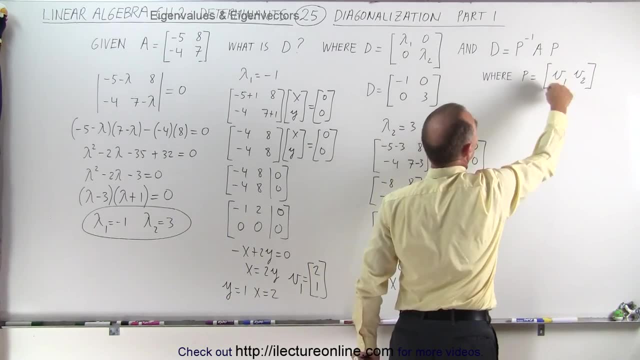 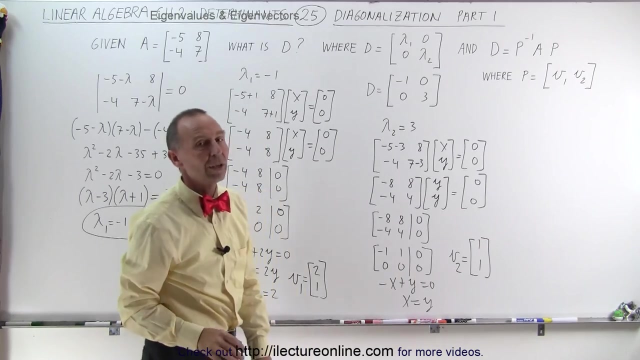 0, 0 zeros everywhere else. that gives us the diagonalized matrix and for the next part, on the next video, we already found the two eigenvectors which we'll be able to plug into this matrix right here, and then allows us to find the diagonalized matrix in this fashion as well. So stay tuned on part two.